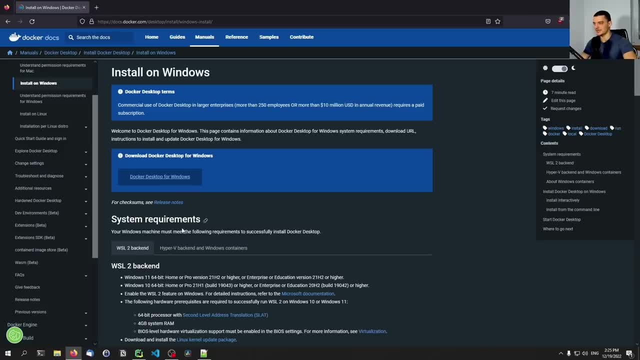 installation process. It's quite simple. you download Docker desktop, for example. you will need to have the Windows subsystem for Linux to back end, or the Hyper-V back end, So one of the two virtualization features or environments. I have a video on the Windows subsystem for Linux. 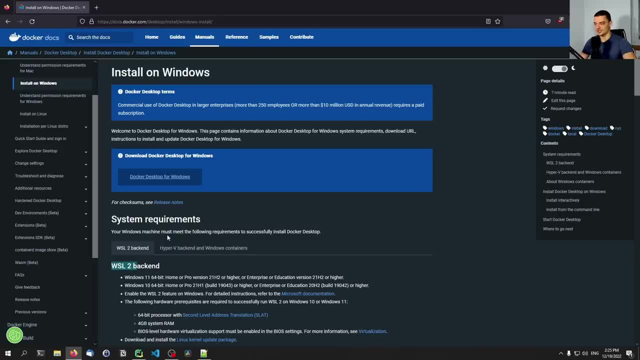 already. So if you want to know how to install it, you can watch that video. Otherwise, you can also just follow the installation guide here on dockercom, But you will need to have Docker installed. This is basically the containerization environment, you could say, And the basic idea of 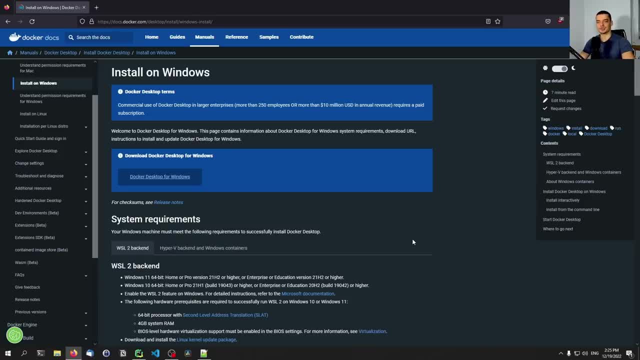 using Docker, or containerization in general, is to package and deploy applications in containers and making everything more consistent and reproducible. So if you have a container, this container will just run. it will just run. It's a virtualized environment, you could say, and it will just run. 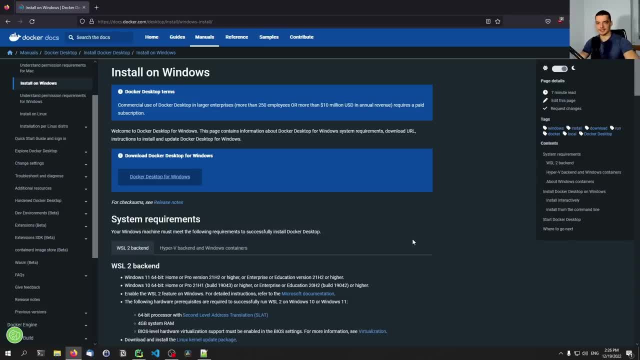 without you worrying about it. So if you have a container, this container will just run. it will just run. It's a virtualized environment, you could say, And it will just run without you worrying about it. So you can package and run applications in those containers And this overall improves efficiency. 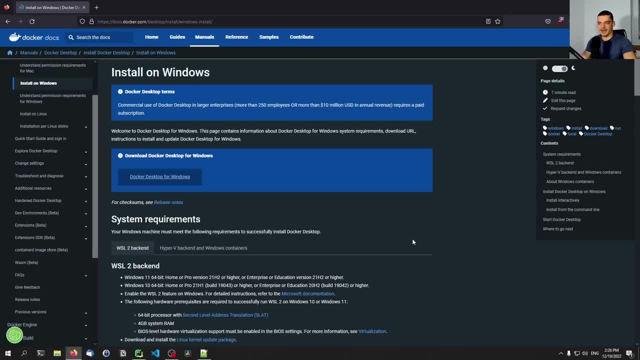 and scalability. So it just makes sense: If you have something that you want to be able to run everywhere, you can just ship it in a container, And if the environment supports running containers, you can just run it everywhere. That's the basic idea of using Docker, of using containerization. 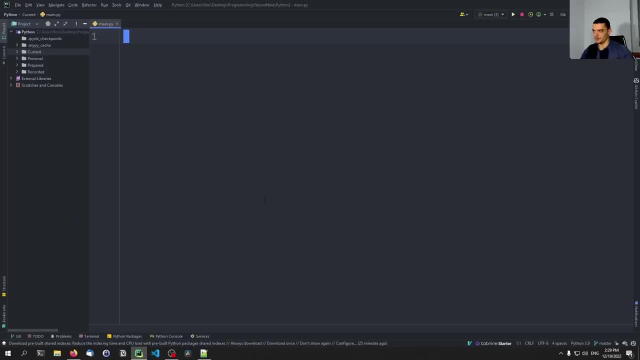 Alright. so once we have Docker installed, we can go to the development environment of our choice, in my case PyCharm, and we can write a simple Python script that we then want containerize, that we then want to dockerize, And in this case I'm going to do two different. 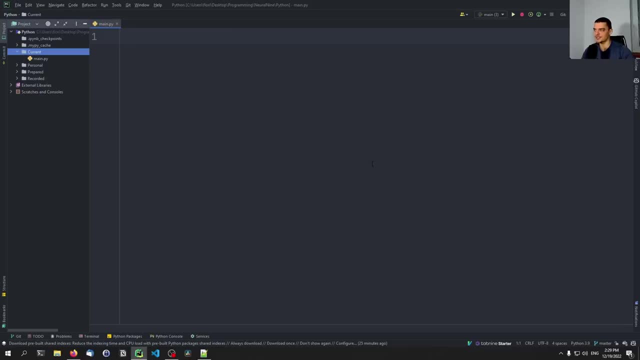 containers. I'm going to do two different applications that we're going to containerize. The first one is going to be a simple Python script that runs a socket, so a server, you could say- and if you connect to that socket it will give you some information. and this information 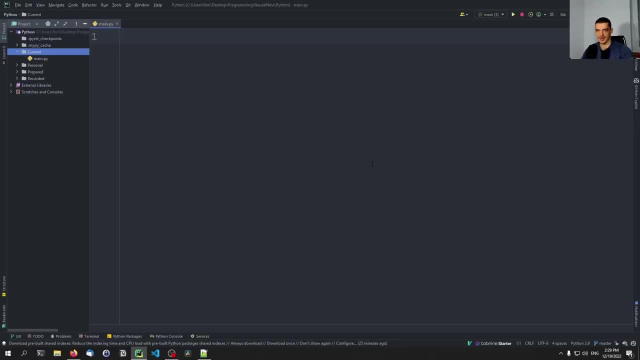 will be taken from a third party module so that we have some dependencies here. So this is not necessarily a useful script. this is just something that works And I'm going to show you how it works in a container. The basic idea is we're going to have a server socket And if you connect to that, 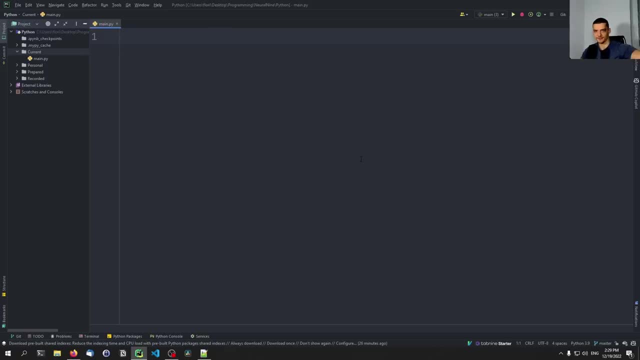 server socket. you're going to get one feature: some data from a data set that is loaded from scikit learn, And the only reason we do that is so that we have a dependency on scikit learn, so that we can see how to install something automatically in the container, Because otherwise we would be. 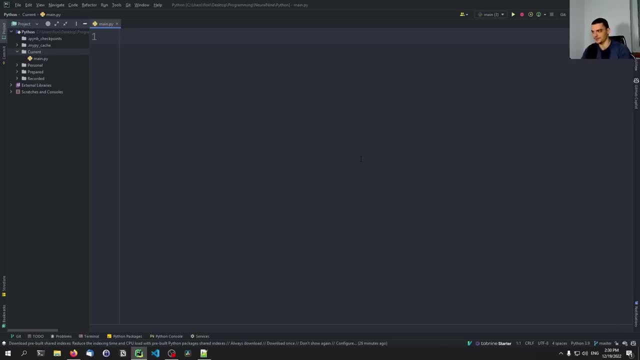 just working with core Python modules, socket and something else maybe. So we're going to start by importing the core Python module time. we're going to import also the core Python module socket And we're going to import the core Python module time And we're going to import the core Python. 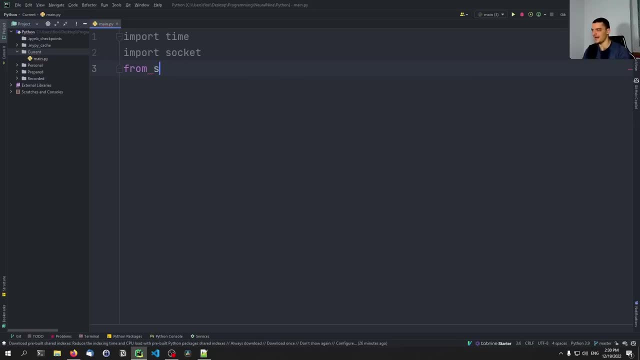 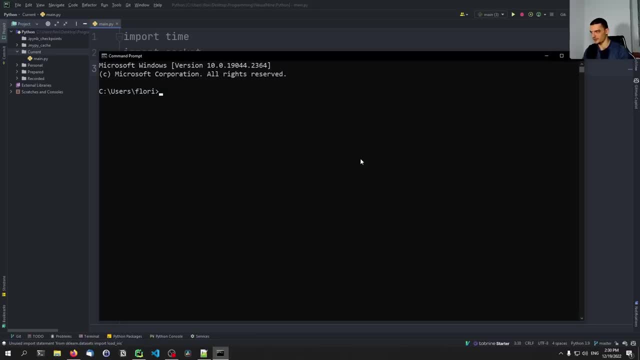 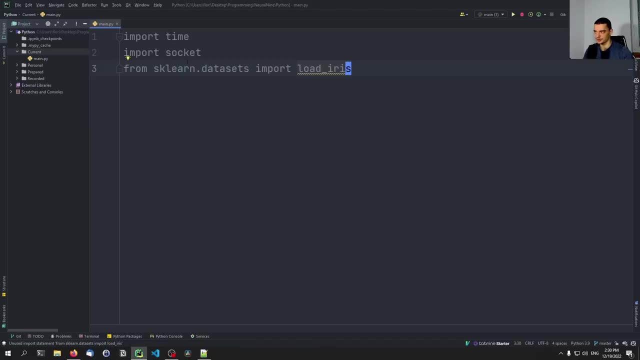 iris. So if you don't have scikit learn installed, you can just open up your command line. you can type: pip: install scikit Learn, like this, and then you will be able to do this import as well. But the good thing is, when you ship a container you don't even have to have it installed on your 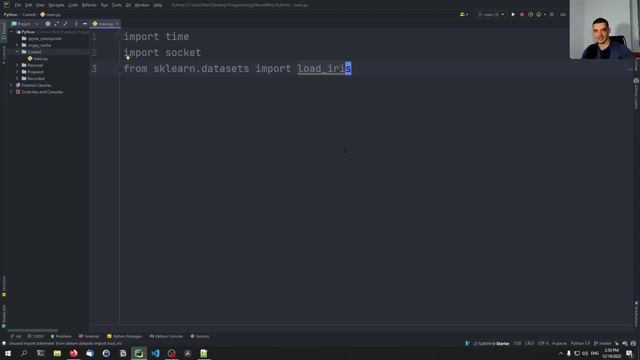 system. So I can actually, once I have the container, uninstall scikit learn so that I don't have this Python library on my system anymore, But in the container it will still know and have scikit learn, So I can still run the features of scikit learn even though it's not installed on. 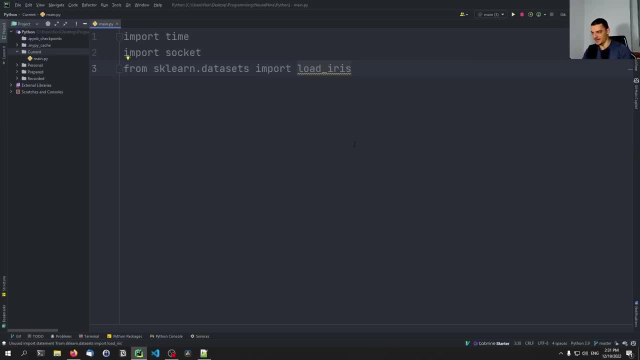 my system because it's running in a container. That's the benefit of this, And the basic idea is to say data equals load iris, to then say server equals socket, socket, socket, internet, socket, so AF, inet, socket, TCP socket, so sock stream, and then server. 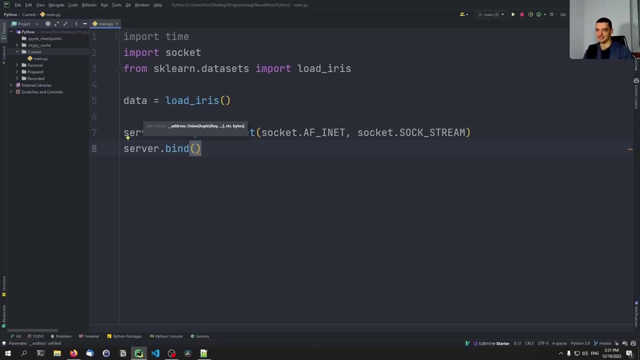 dot bind. Now this is here important. we need to bind it on a special interface here, on a special host here, which is the zero in string, of course, in quotation marks, of course, 0.0.0.0.. So we're. 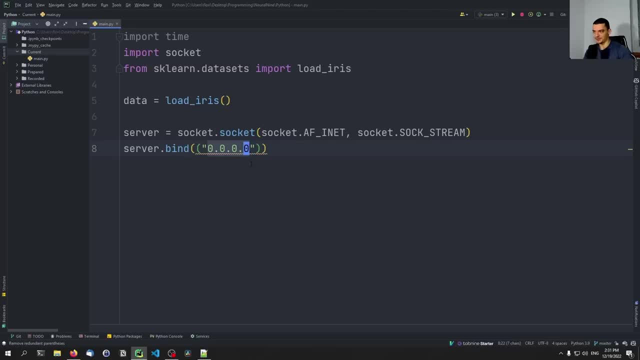 not hosting this on local host. we're hosting this on this IP address, which is important for the Docker container, And we provide a port, for example, four times nine. So this basically means the server is now listening on this host, on this port, And now we can say server. 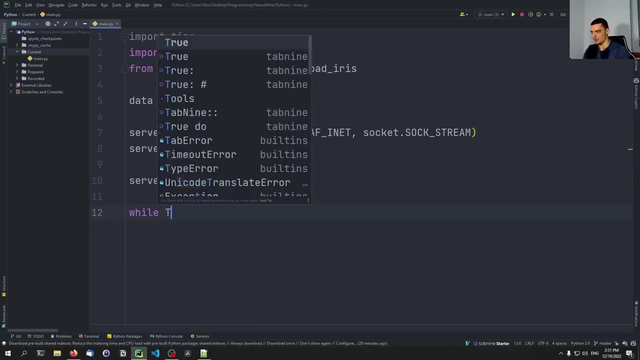 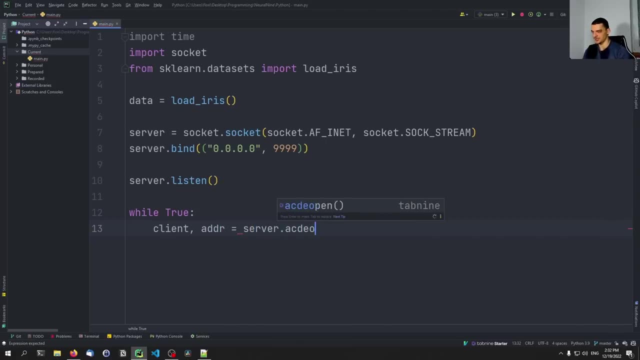 dot listen, to actually start listening, And all we're going to do is we're going to say: while true client and address is going to be equal to server, dot accept. So we're going to accept all the time incoming connections. then we're going to print connection from and we're going to say that the 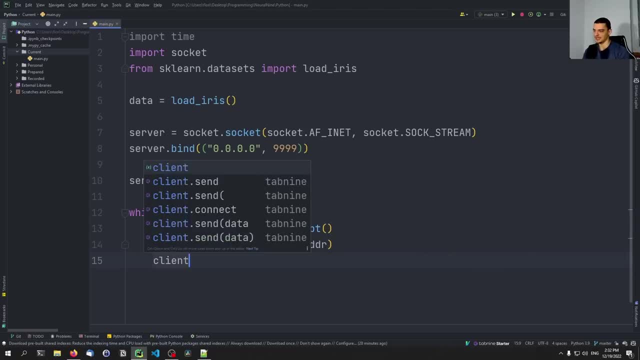 address just connected. then we're going to say client sent, we're going to send something to the client, like you are connected, And then we can also add a backslash And because on the other side, in this case for the 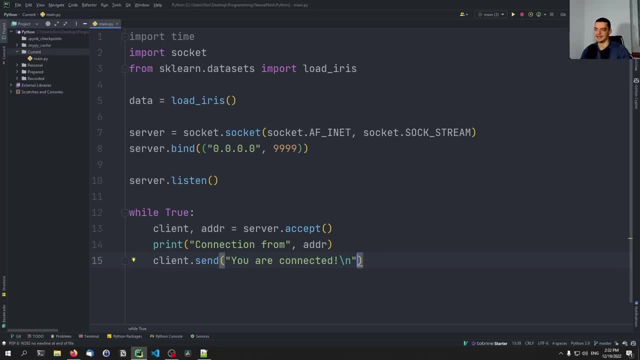 demonstration. I'm not going to write another Python script. I'm going to run a telnet client And because of that we're not going to use the print function. So it's not automatically going to do line breaks, which is why I'm going to send them right away. So I'm going to send your connected. 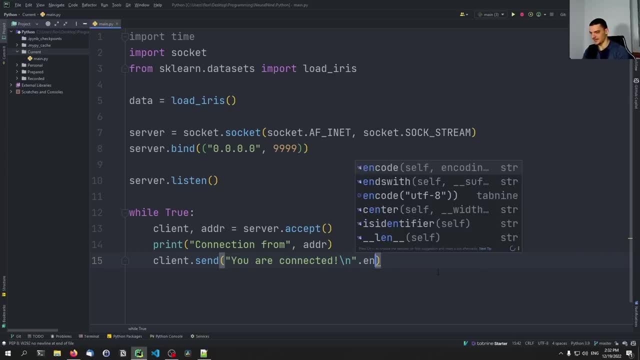 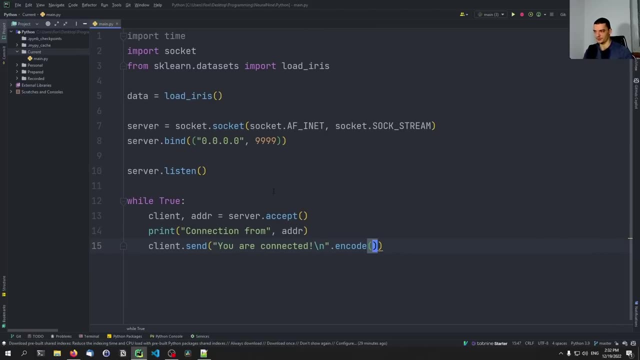 line break, And then this needs to be encoded Again. the specifics of what we're coding here is not too, are not too important, Because the focus is not on this script we're actually building. the focus is more on the containerization. 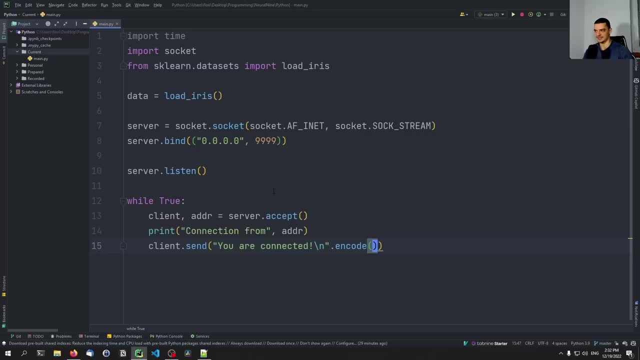 And we're building the script to have something that is listening on a host And that is using third party packages. That's the basic idea. You can also feel free to use another example if you want to. So client sent, and what we're also going to send here now is we're going to send the first. 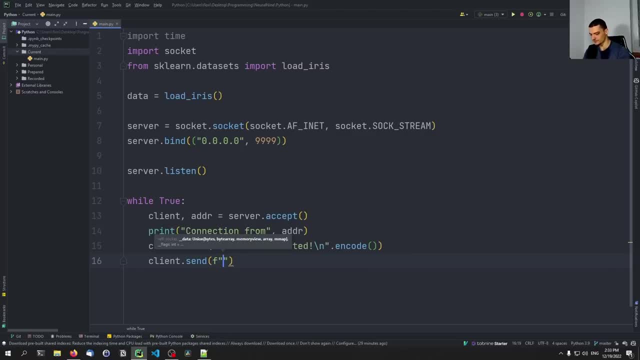 column of the iris data set. So we're going to say data, of course in curly brackets we're going to say data, and then we have the key data And here we have everything from the first column, So the column with index zero. 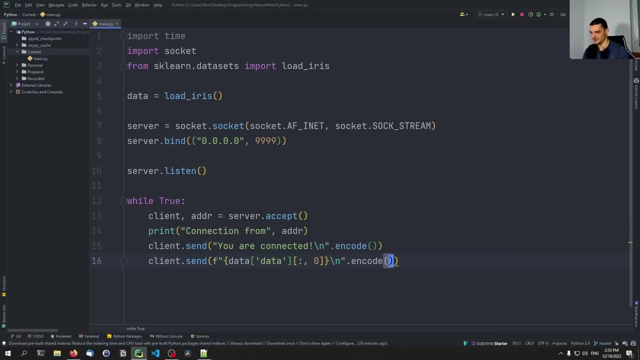 And then we're also going to add a backslash and we're going to encode this, And then we can do something like time, sleep two seconds or something, and then client sent: you are being disconnected, or something like that. And of course this needs to be encoded as well, because 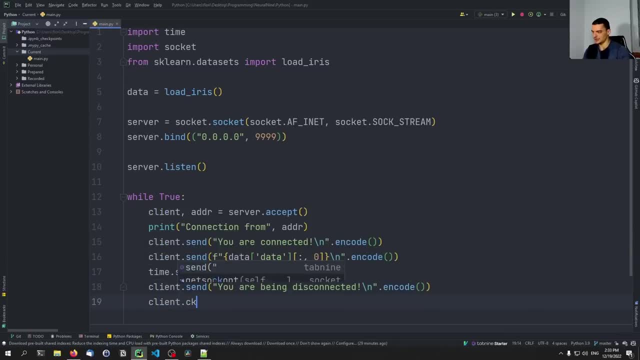 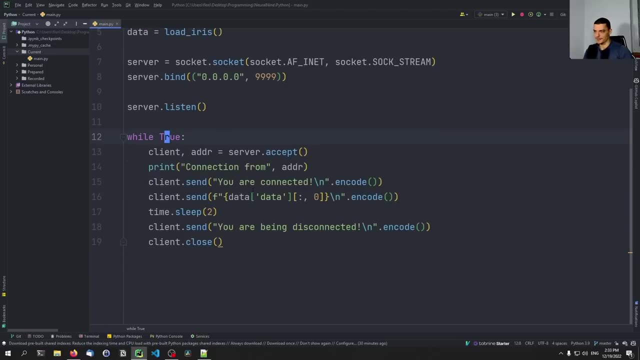 we can only send bytes via sockets, And then we're going to close the connection with a client And we're going to listen for new connections, So we're going to accept the next connection. This is an endless loop. So that is the script. we can actually run this now without a docker. 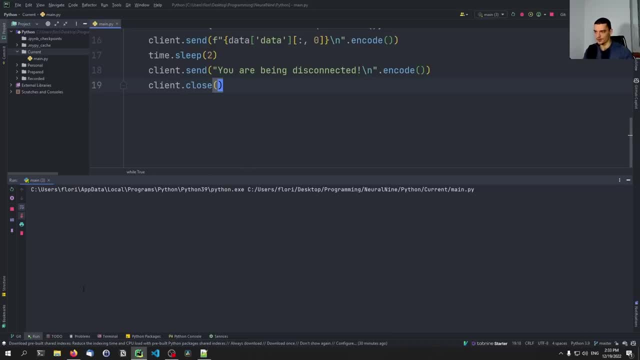 container. So it's just listening. we can then use a telnet client Now on Windows. if you're using the telnet client or if you want to use the telnet client, this is a deprecated feature, an insecure feature, you could also say so. it's disabled by default. if you want to do this for just debugging. 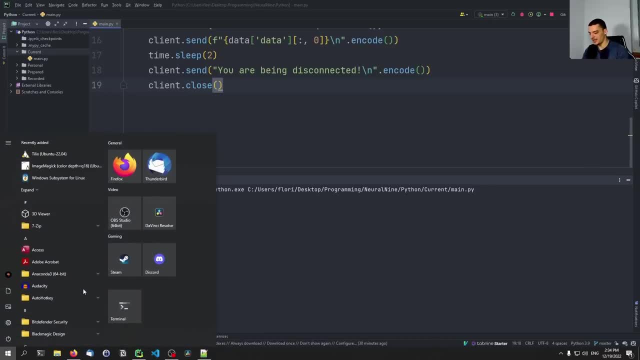 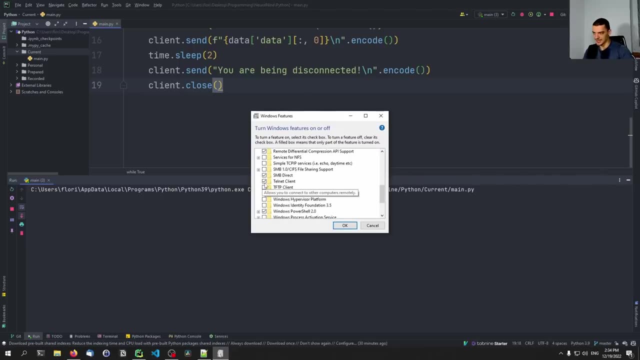 or demonstration purposes or just playing around with it. you can go to features, So turn Windows features on or off, And you can scroll down Here to the telnet client and check it, and then you will be able to use telnet in the command line. 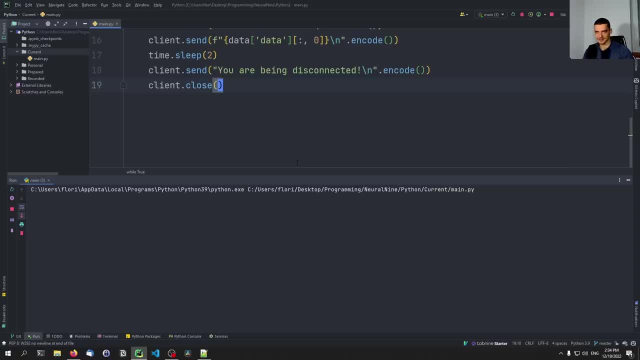 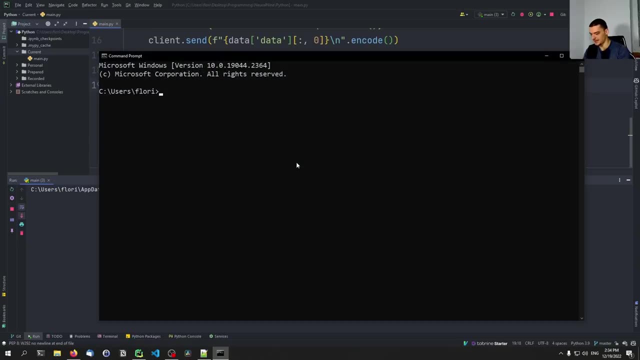 On Linux it's simpler. If you're doing this on Linux you can just use net, cat, So NC, to connect to that host and port. And we're going to just open up the command line now And we're going to say telnet. Now I'm not sure if this already works with a host we provided, But let's see if I. 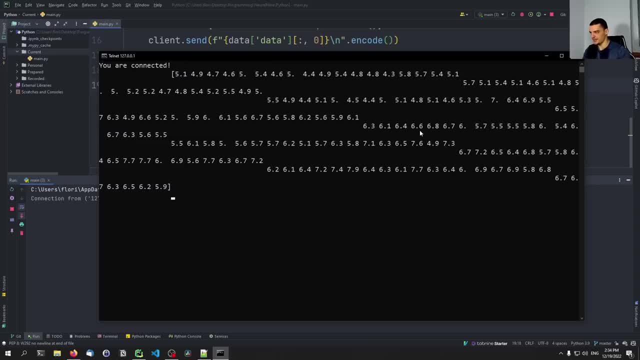 connect to localhost port 9999.. There you go, you are connected, we get the data. Again, doesn't matter what the format is, we're just getting the data. So we're going to go ahead and connect to the docum it is. we're just getting some data here And that is basically it. So this is how. 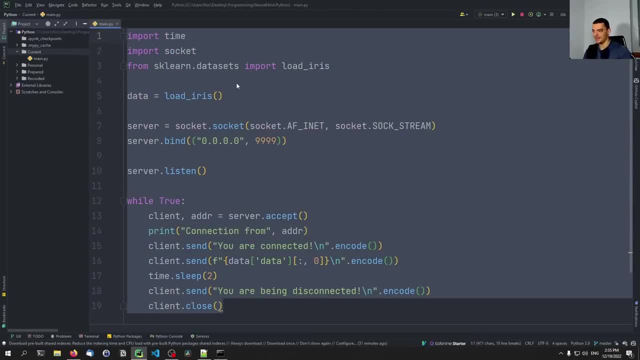 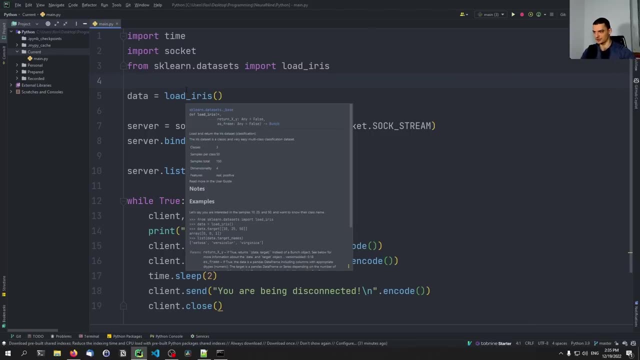 this works And we want to now take this and reproduce the functionality in a Docker container. So we want to have a container that we can just chip to someone. this person might not have scikitlearn installed. they will still be able to get the data from scikitlearn because in the 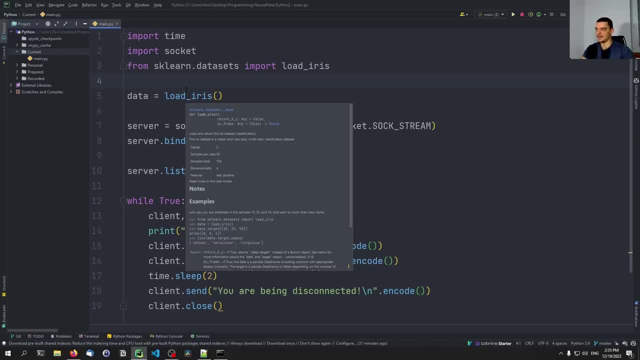 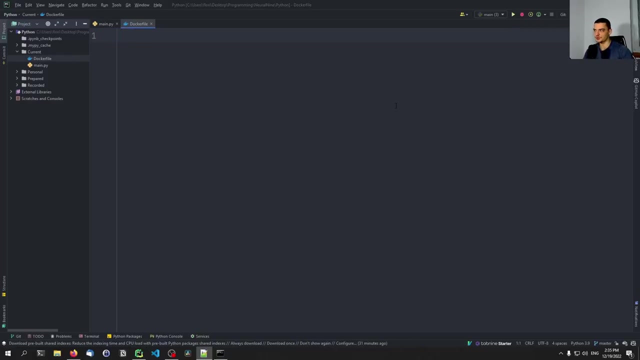 container, we will have all the dependencies and everything we need, And this is done with Docker and with a so called Docker file. now is we create a new file And we call this file Docker file, with a capital D, And you can see already in Python we get this icon, this Docker icon, And what we're going to provide here. 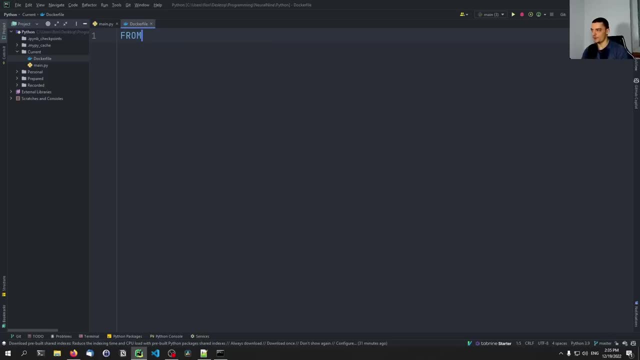 for this script is quite simple. We're going to say, from in here, we need to provide a Python version. So it's going to be Python, in my case, 3.9.. This is the version I'm using. you can. 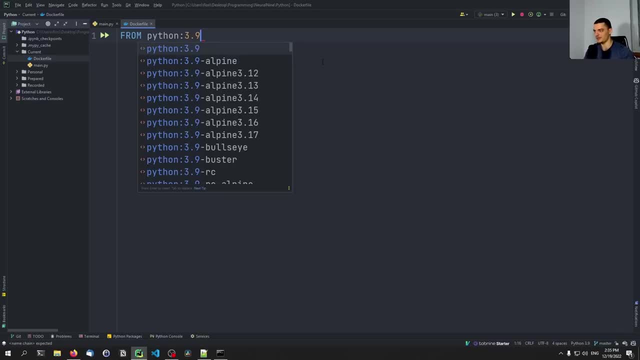 of course also provide Python 3.10, 3.11, or some stuff like slim or certain snapshots from previous or something, But I'm just going to go with a classic 3.9.. And then we're going to say we want 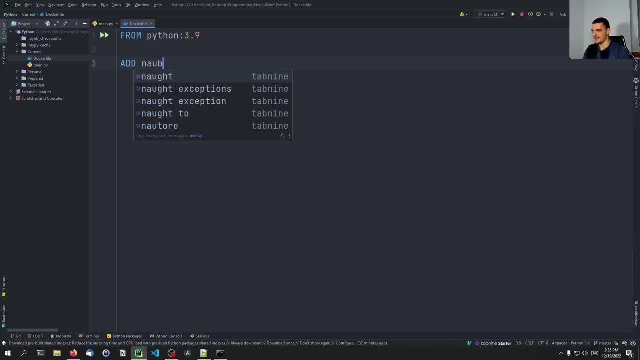 to add some files, And the only file that we want to add here is the main dot py file, And we're going to add it, to dot so, to the current directory. And then we're going to just run a command, And this command is going to be: pip install, scikit learn. So this is why I wanted to use a third. 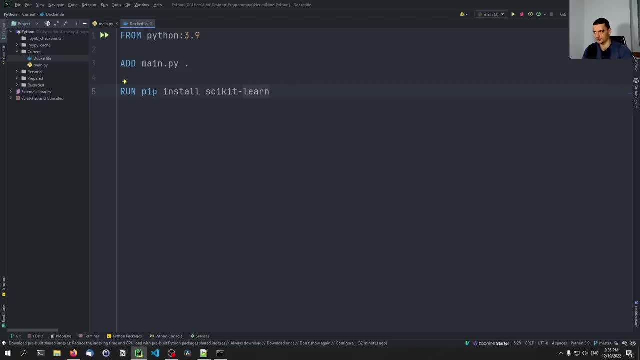 party package, Because if you don't use a third party package, there's no need to run pip install. But by specifying this, by specifying run pip install, scikit learn this is going to run this installation command when creating the Docker container, And in the Docker container we will then have scikit learn. That's. 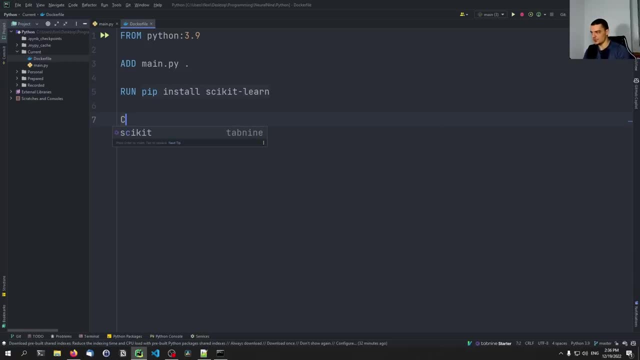 the basic idea. And then the last thing, quite simple, is: we're going to execute the command, and the command is going to be Python, And then the second keyword is going to be dot slash, main dot py. So we added main dot py to the current directory And here we're just running it. 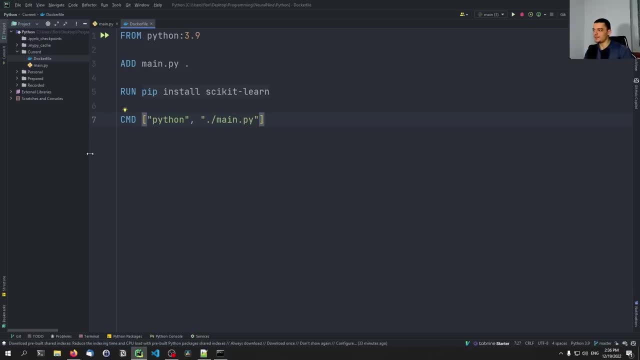 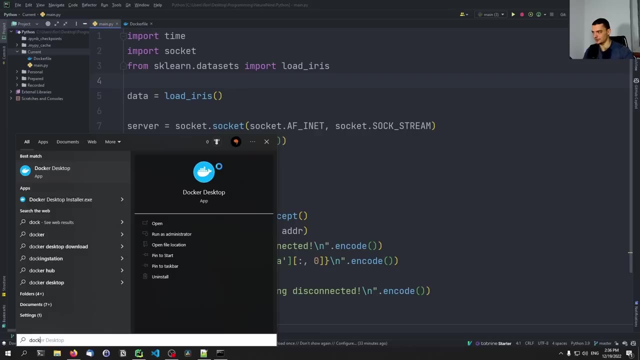 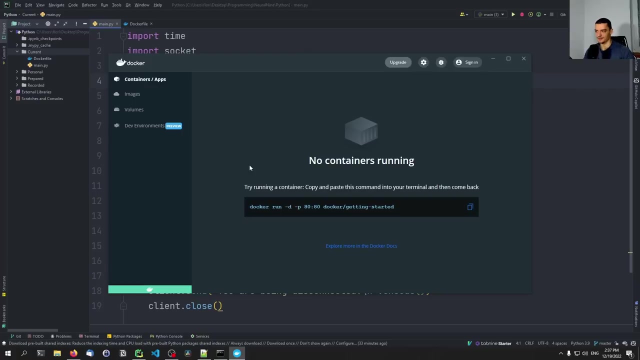 that's the basic idea, And in order to now build this container, we need to have Docker installed. As I already mentioned, we need to have Docker running as well. So if you have Docker installed, you should have this Docker desktop app. you want to run it And once this is running, your you have the Docker daemon running. So 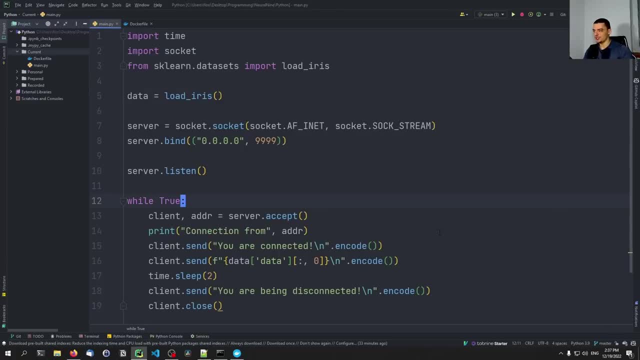 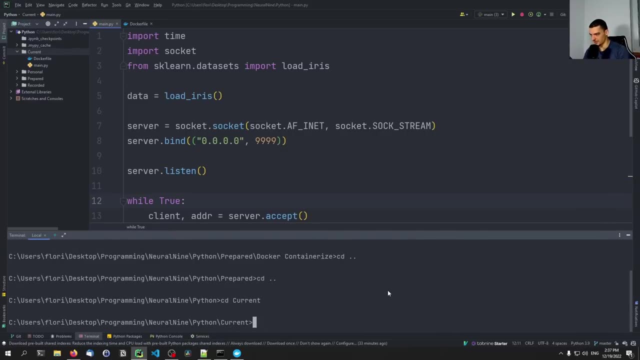 Docker is running in the background so you can use it, And all you need to do now is you need to open the terminal or the command line. We're going to navigate to the current directory here And in the current directory. I hope you can see. 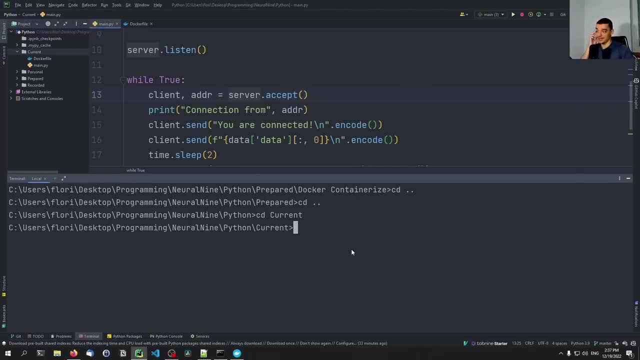 this. well enough, I'm going to zoom in a little bit. in the current directory we're now going to run the command that is necessary to build a container, And this again only works if Docker is running. So what we're going to do here is we're going to say Docker built dash T and then 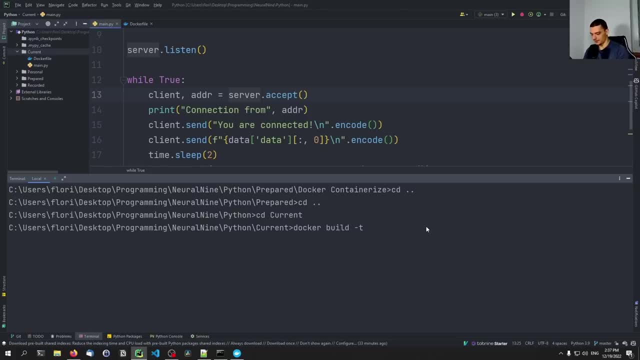 the name of the container. For example, I don't know, Iris, Iris dockerization or something like that, And we're going to specify the dot to again target this current directory for the build process. I'm running this and then the Docker. 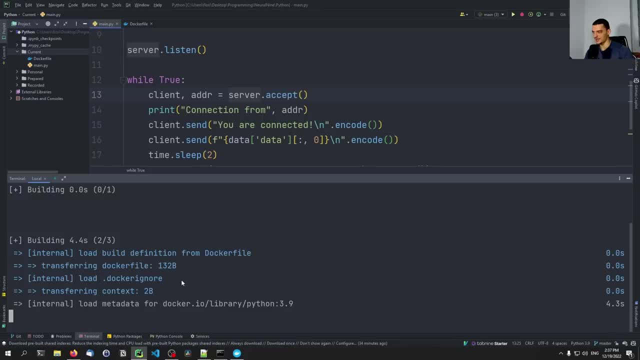 container is being built. you can see here to building process is running. we will also see. I think that it's going to install scikit learn. there you go to run pip, install scikit learn. We also added main, not P? y. you can see how all this is happening And then after a while, 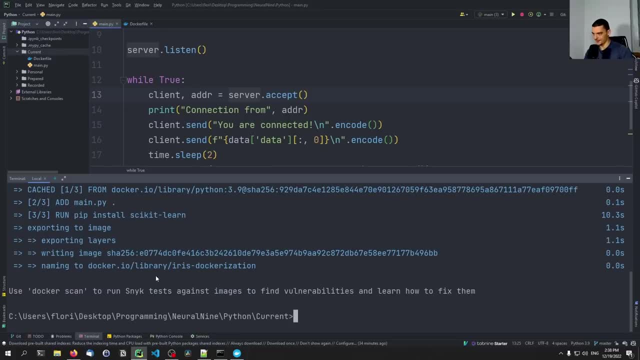 it will be done and we will have the Docker container ready. So now we have this Docker container, it has this name: Iris. what do we call it? Iris dockerization, And we can now run this container as well, by just changing their name. This is the running container. We can now run this. 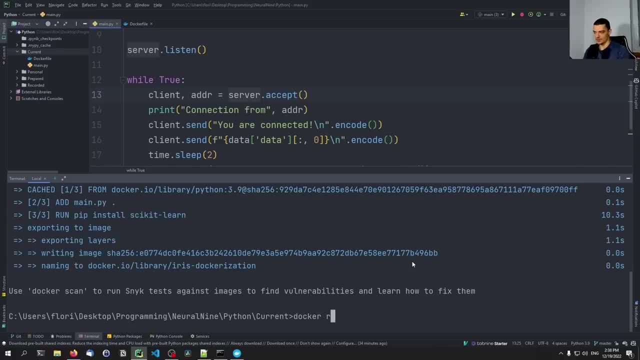 container vi by just saying Docker, And then we can say run. And if we want to use ports, if we have some networking stuff that is running, we need to map the ports as well. So if you don't have ports, if you're just running something, you don't need to specify anything network related, obviously. 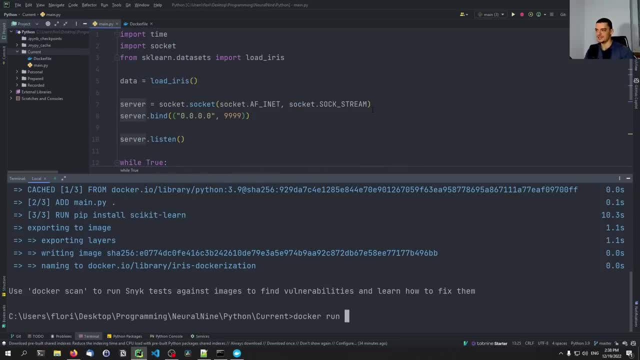 But if you have, in this case, a server listening on a certain port, you need to map that port to a port on your system. So you want to say dash P and the port 9999 shall be mapped to 9999. Otherwise, 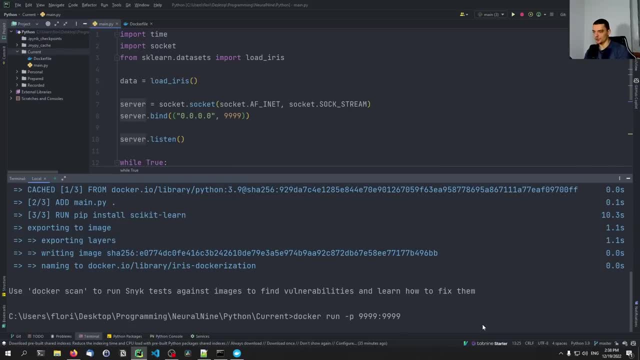 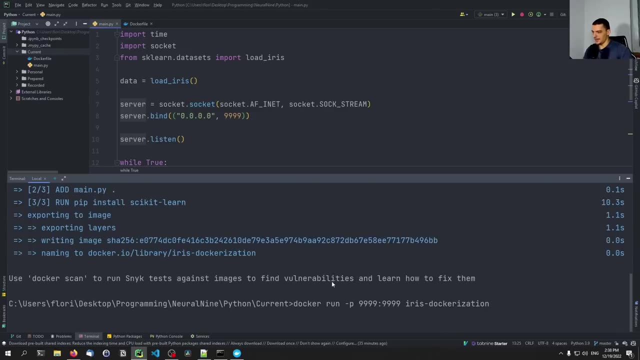 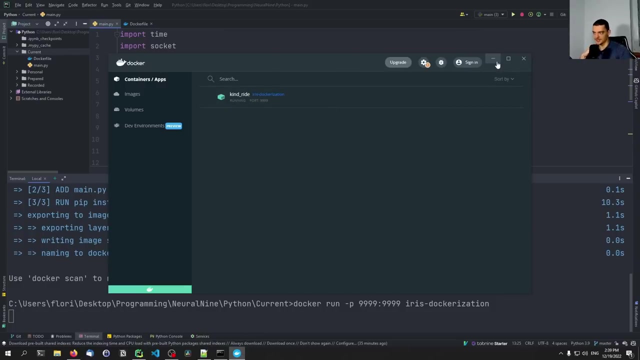 it won't work. And then we also want to say, okay, what are we actually running? We're running the iris dockerization And then this is running. you can also see here: iris dockerization is running in the Docker desktop graphical user interface environment. And now, even though 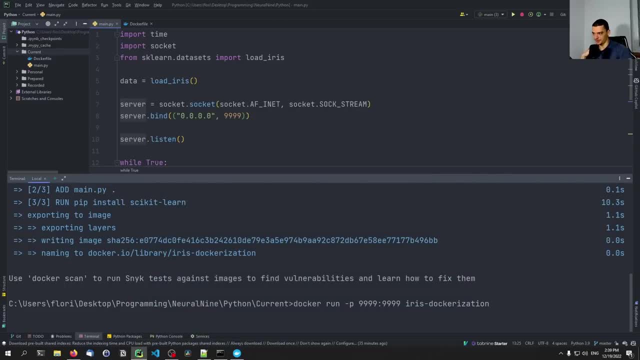 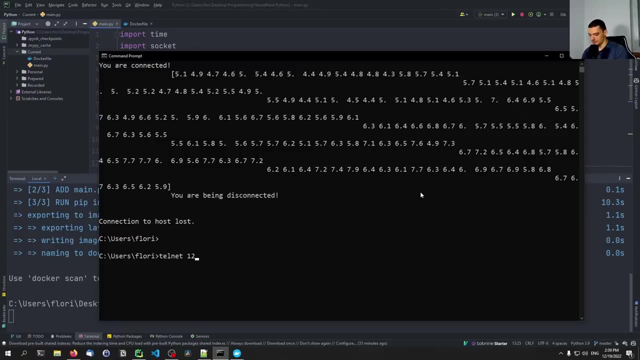 nothing is running in PyCharm. even though I'm not running the actual script here in PyCharm, I will still be able to just say telnet 127001.. There you go. So I can still get this connection, even though it's only running in the. 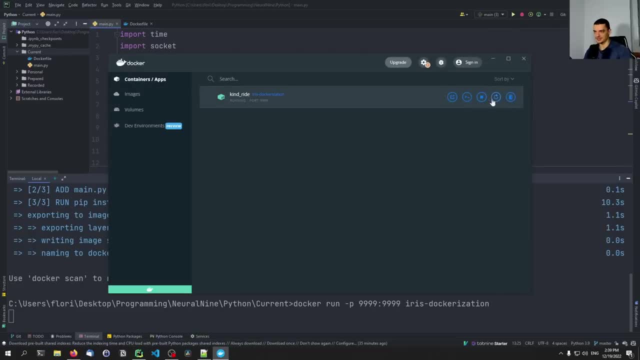 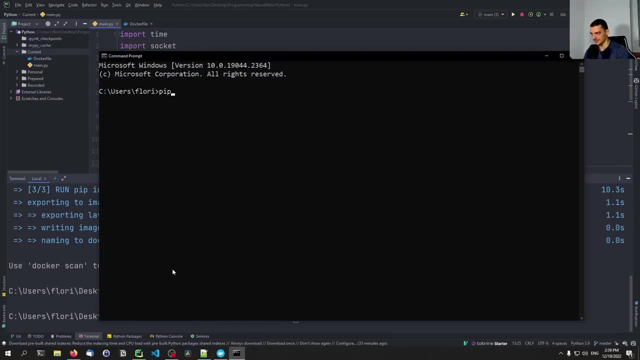 Docker container. So you can see that this works. And I can also. this is the most interesting thing: now I can delete this. now What I can do here is I can also go to my command line and say: pip- uninstall scikit learn. So this removes scikit learn from my system, And you will see that this 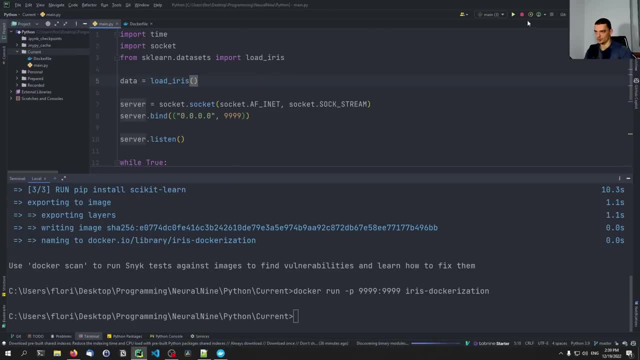 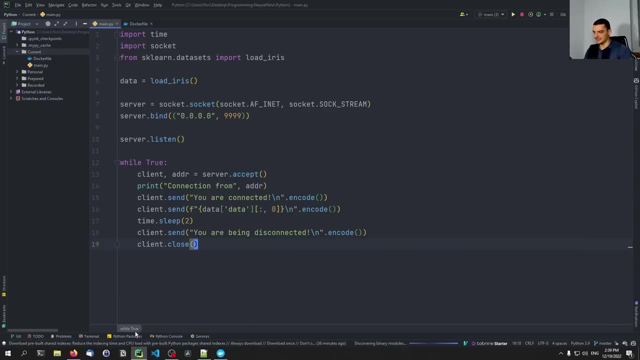 is the case, Because I will not be able to run this script anymore. I will not be able to run this because it says no module named scikit learn, So I don't have it on my system. However, I can still go into the command line and execute this last command to run the iris dockerization. I can. 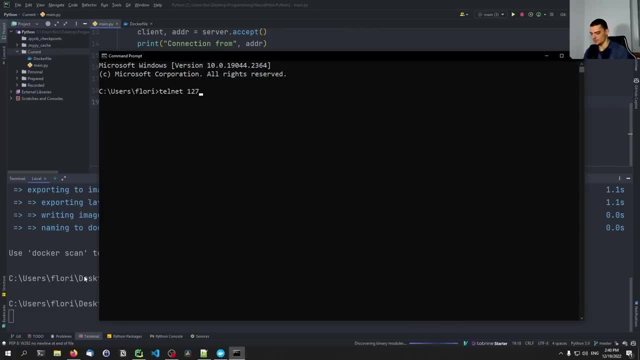 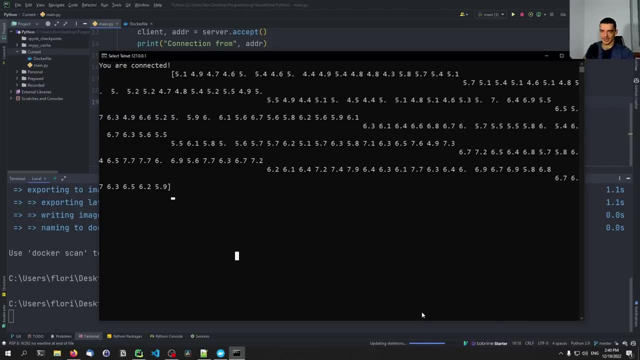 still open up my command line, I can still connect telnet 127001 for localhost And you can see that I still get the data because in the container, scikit learn is present, even though it's not active on my system, even even though it's not present on my system. 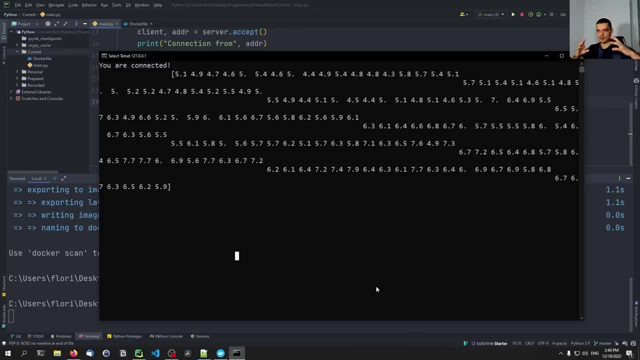 I can do everything because in the container I have this reproducible environment. I don't need to worry about dependencies, I don't need to worry about installation. everything in the container is there And I just have to run it and I can use it. That's the benefit of using Docker containers. 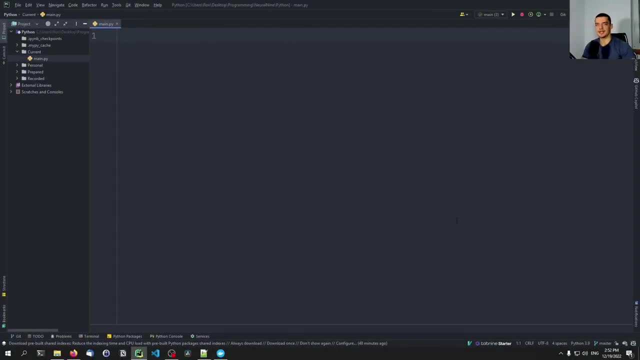 Alright, now let us move on to an additional example. We're going to containerize a fast API application, And this is oftentimes the sort of hello world example for beginners when it comes to Docker isation and Python. If you Google how to containerize Python applications using Docker, you will see that it is still working. 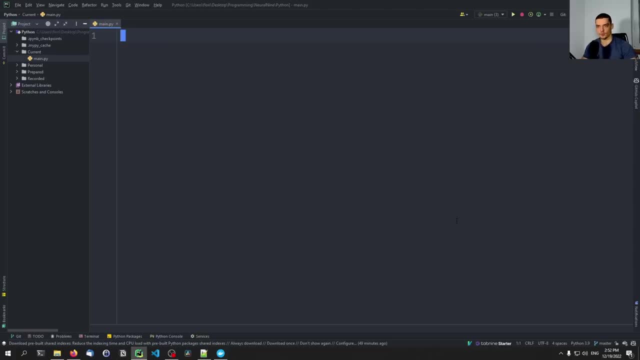 oftentimes find examples using FastAPI, And because of that, I wanted to include such an example here as well. And for those of you who don't know, FastAPI is a simple framework that allows us to easily build REST APIs. I have a video on it as well, And the basic idea is you. 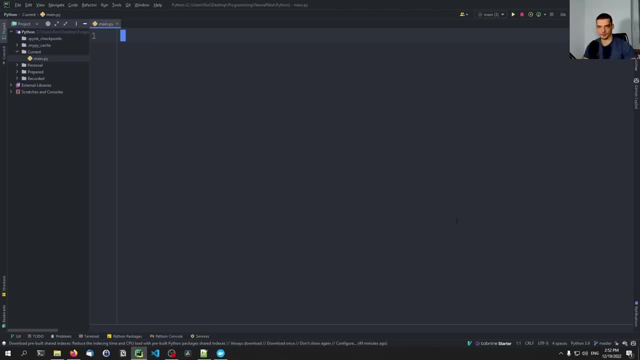 specify a couple of functions, you map them to a certain endpoint and then you have your REST API without having to use full-blown web frameworks like Flask or Django. FastAPI is, as the name already says, the best library to build a simple API fast, And we're going to build such a simple. 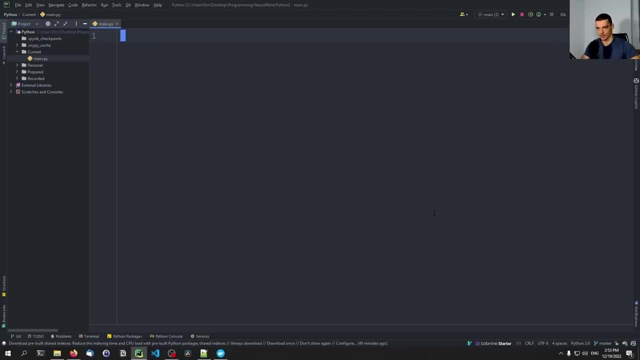 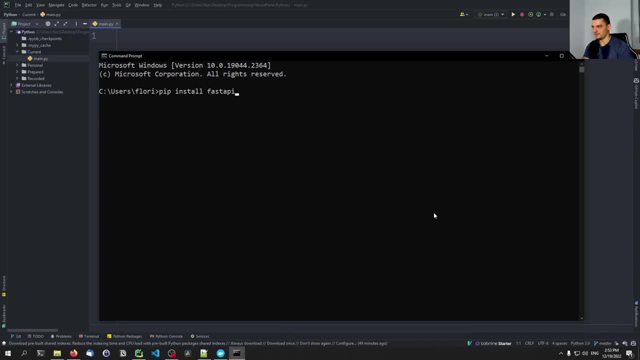 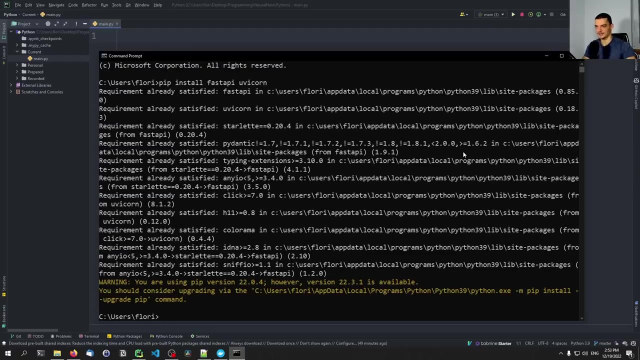 API, now with just a single endpoint, and we're going to containerize it using Docker. So, in order to be able to work with FastAPI, we're going to use pip to install FastAPI and UVCorn, even though I'm not sure if UVCorn is not automatically installed using FastAPI or by installing FastAPI. 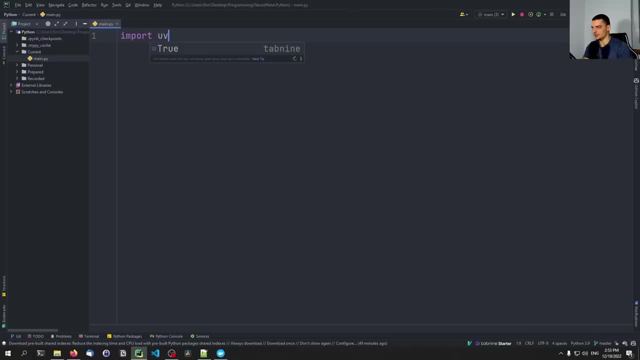 But you need those two things and then you're going to have to import UVCorn also from fast API. import fast API like this. then we're going to create a simple application by saying app equals fast API, and then we're going to provide just. 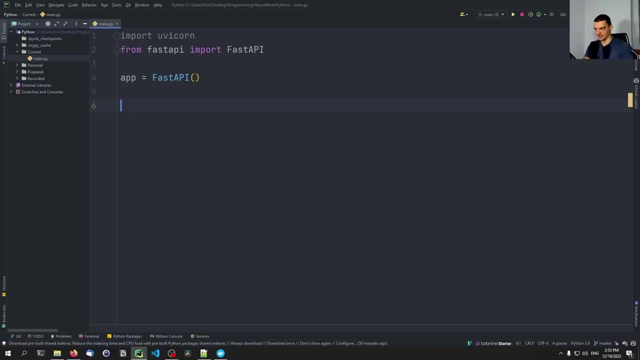 a single endpoint, just so that we have something. and then we're going to containerize this whole application and we're going to call the function here main function, even though, okay, this name is probably misleading. let's call it central function or something. you can call it whatever you want, and we're 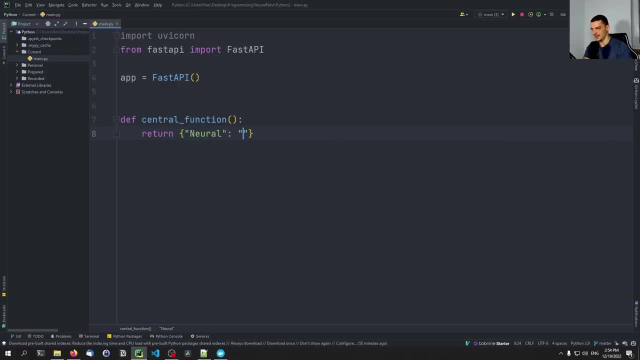 going to just return a dictionary here that says neural is the key and nine is the value. so this is our JSON object and in order to get this response you will have to send a get request. so app dot, get to the root endpoint, so just slash. that's the basic idea. and now, in order to run this, what we do is we say if 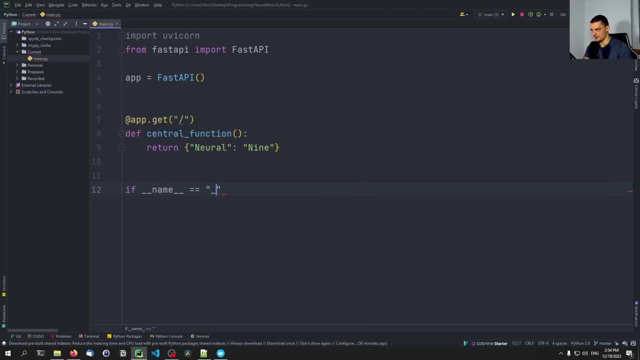 underscore- underscore- name equals underscore- underscore, main underscore- underscore. if that is the case, we're just going to say UV corn dot run and we're going to run the app. we're going to specify the port 8000 and we're going to say that the host is again zero point, zero point, zero point, zero, and that. 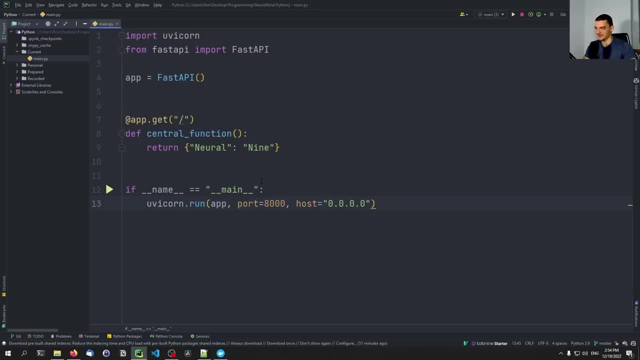 is basically it. so this is our fast API. of course, you can make it more sophisticated. you can have multiple different endpoints with multiple different HTTP methods supported, and those do some data science work or something. but this is the most basic example which we're going to use here. 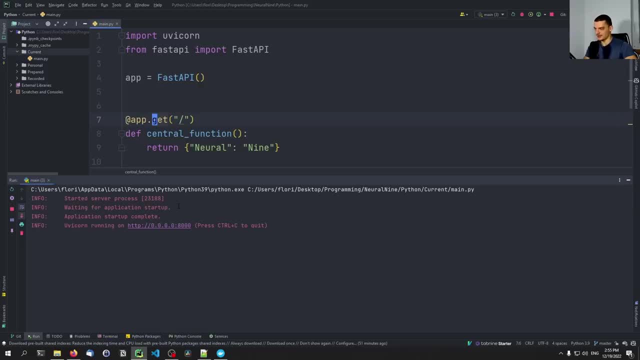 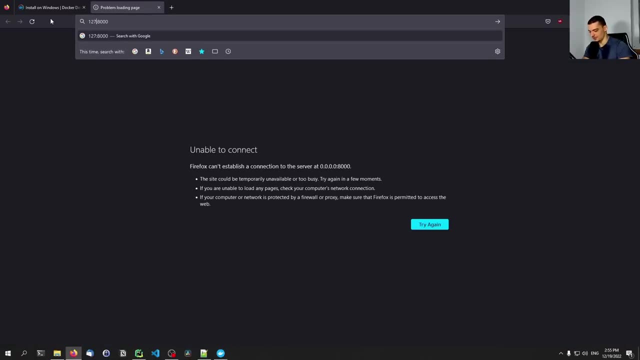 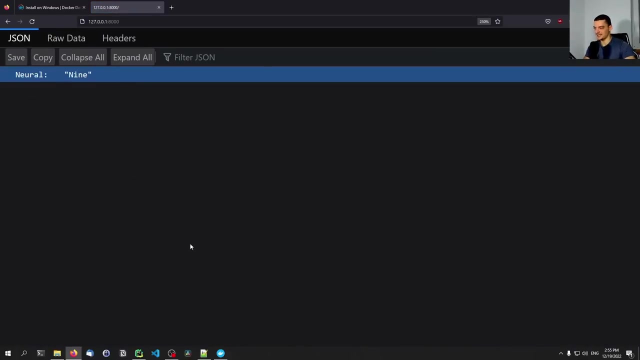 for the containerization. I can just run this now and then you can see that this is running now on zero, zero, zero, eight thousand. I think I should be able to access it on localhost. there you go and you can see I get neural and nine. that is our API now, and we can containerize this API with docker. so I'm 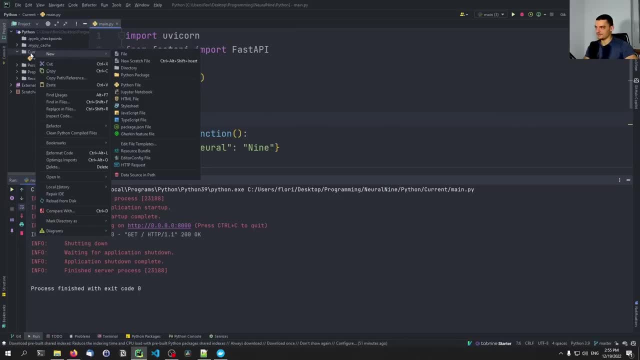 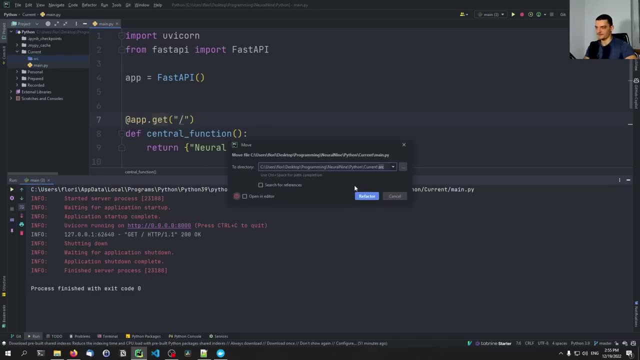 going to close this now, and usually you have a structure that is not just a main file. you usually have something like a source folder, so you have SRC and then this main file is inside of SRC, for example, and then we're going to run this. we're going to also have again a docker file, so we're going to have a simple. 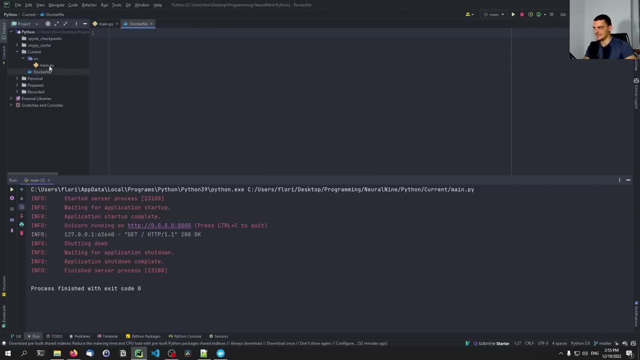 file- docker file- with a capital D again, and in addition to that, this time we're going to provide also a requirements txt file, so that we have a file with all the modules needed. so we're going to create a new file here, requirementstxt, and the basic idea is: here you just list all the modules, all the dependencies of your application. 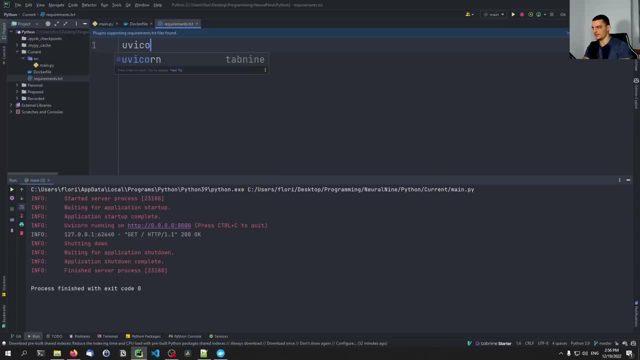 in this case uvcorn and fast API. so just uvcorn and fast API. if you want to have a specific version, you can just say equals, equals and the version number. but we're going to just specify the names now. and, of course, if you're using pandas or scikit-learn or matplotlib or anything, you 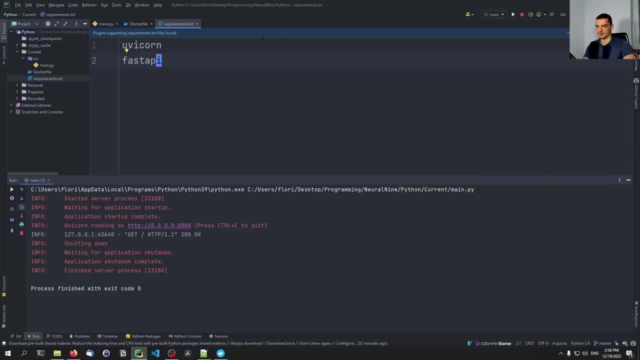 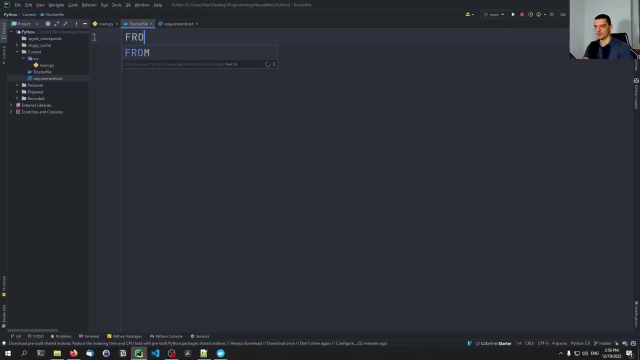 just put it into into the requirements, and then you have to install it, of course, with a certain command in the docker file. but we're going to do this here. so, again, we're going to start with a simple from python 3.9. we're going to then say: the working directory is going to be- let's call this, I don't know- neural. 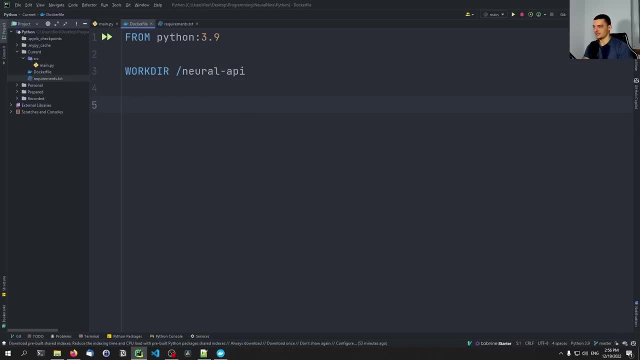 dash API and this just specifies the working directory, the context of this whole thing, and we're going to then copy the requirements txt file into the current directory and we're going to also copy the source folder. in this case there's only one file in the source folder, but 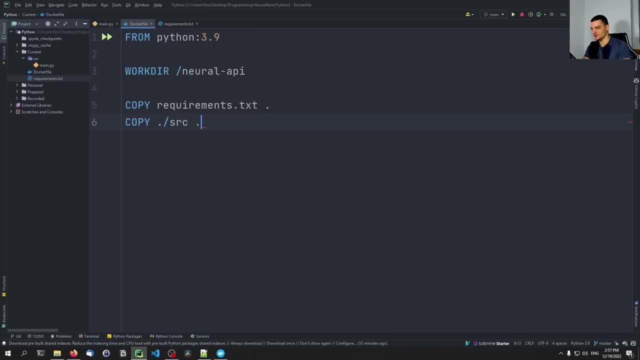 in general. we're going to copy the whole source folder and we're going to say that we want to put it into another folder that has the same name. so we're getting this folder here and we're putting it into a new folder that has the same name. that's the basic idea here. we're using the copy command for this and then 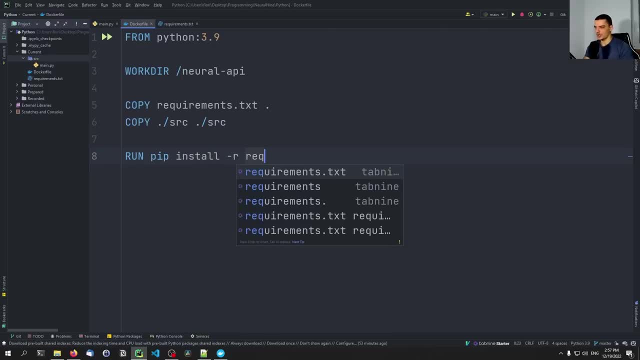 we just say: pip install dash r requirements txt, because this file is now added to the current directory. we can just use it in the pip command and once this is done, we just have the same command. so we just specify again and then dot, slash, source, src, slash, main, dot py, and this is the docker file that we need here. 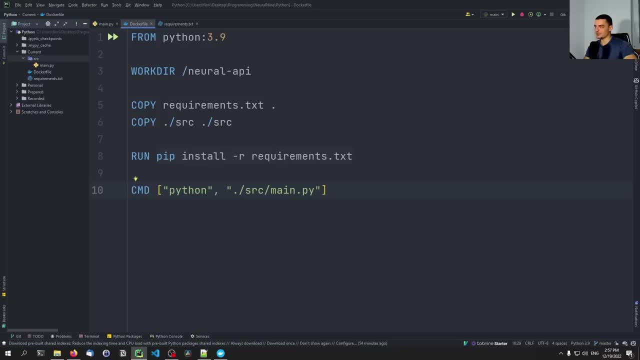 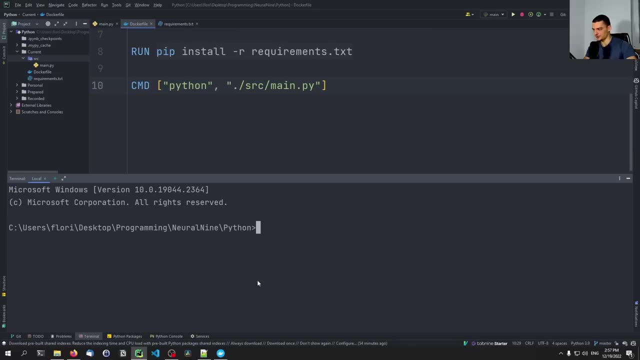 now what we can also do is we can, um, we can basically use the same build command now, but we can also specify a name. so I can go into the terminal here, I can navigate to the directory and I can say again: docker, uh, built dash t, neural dash. 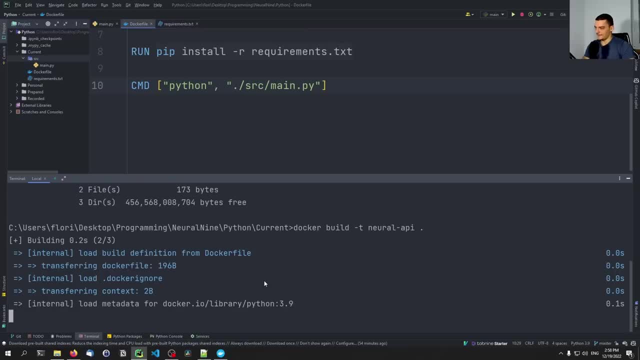 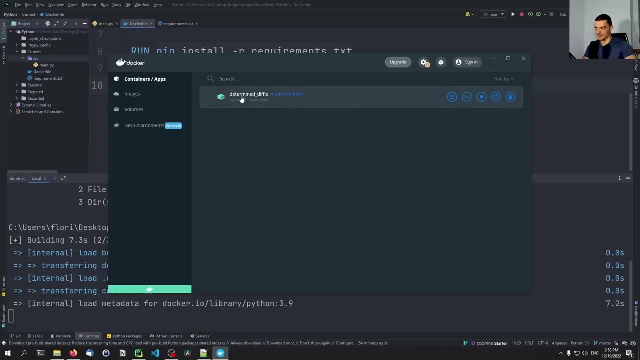 api, for example, um, and then we're going to, when we're running this, we can specify a name. so if you go to the docker desktop here you can see it just assigns a random name, determined diffy or or dify, diffy, I think. uh, and then the actual container. but we can also specify such a name. 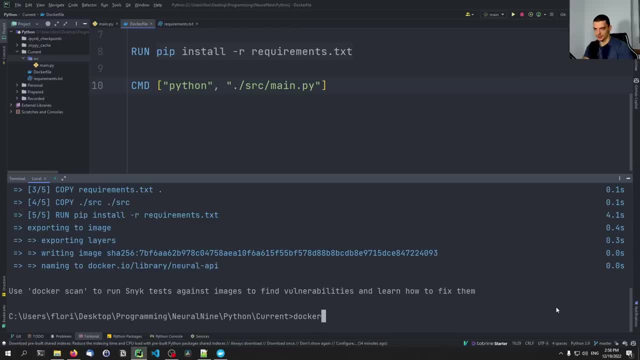 manually. we can just go ahead and say uh, docker, and then again run, we're going to map 8000 to 8000 again. since this is a, an api running on a port, we need to map the port again, this port here, um, and then we can just specify dash, dash name and we can say I 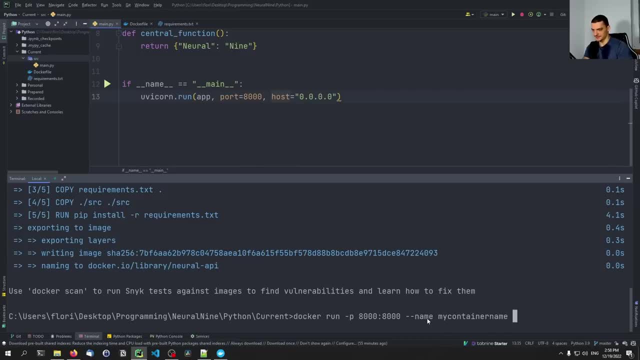 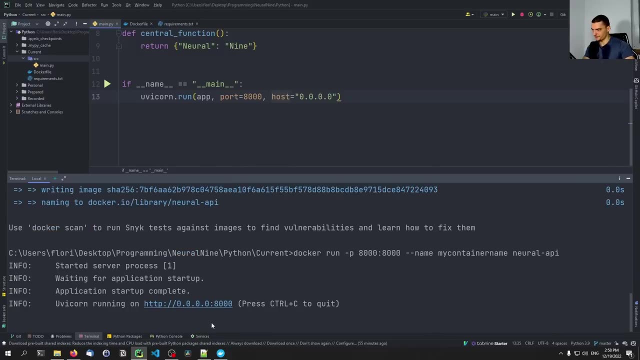 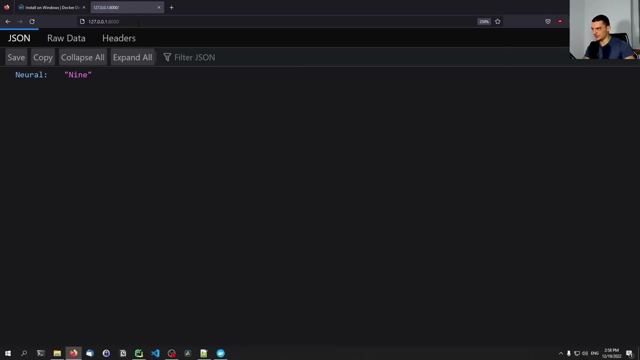 don't know my container name, and then I can specify neural api and I think I didn't forget anything. so that should work. there you go, you can see it's running and here we can see my container name, so I can just use it from here. now I can go again to localhost and you can see the api is.